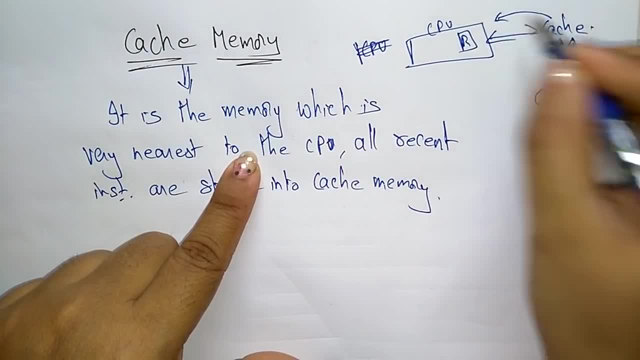 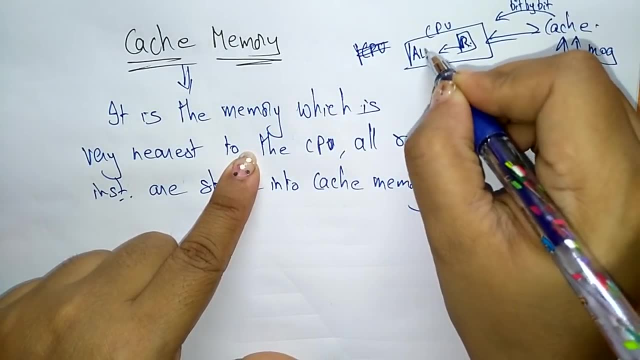 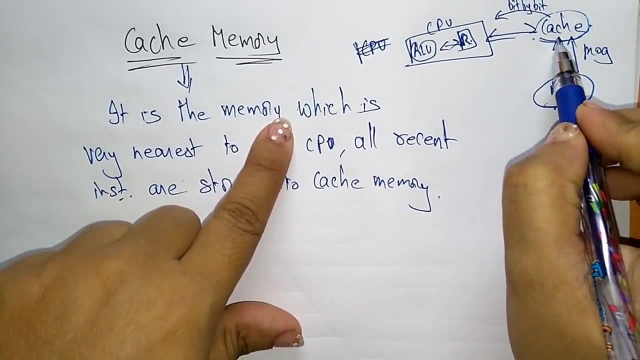 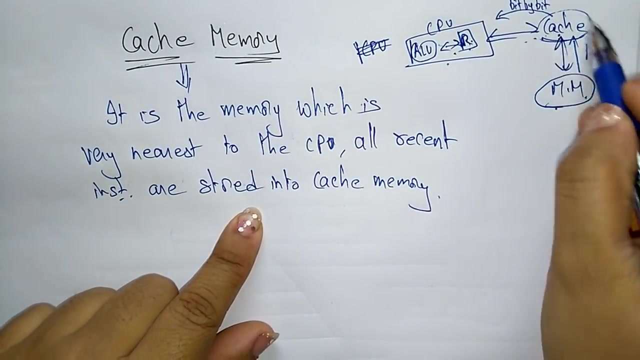 So the cache will send a bit by bit to the register and the register will send to ALU to perform the operation. So the cache memory, this cache memory is very nearest to the CPU. So which is very nearest to the CPU and all recent instructions are stored into the cache. So, whatever the recent instructions that the CPU has to be performed, those instructions are stored into the cache. 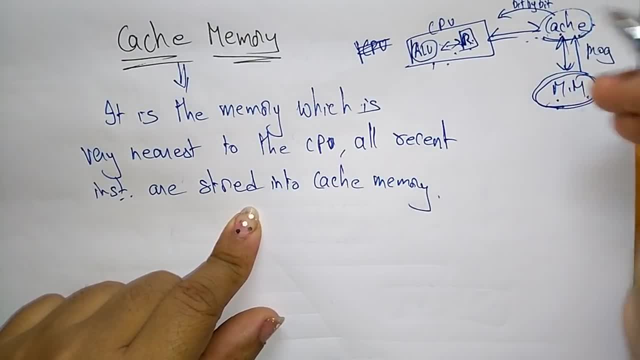 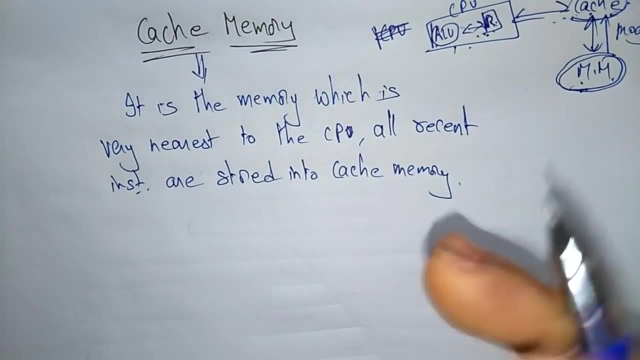 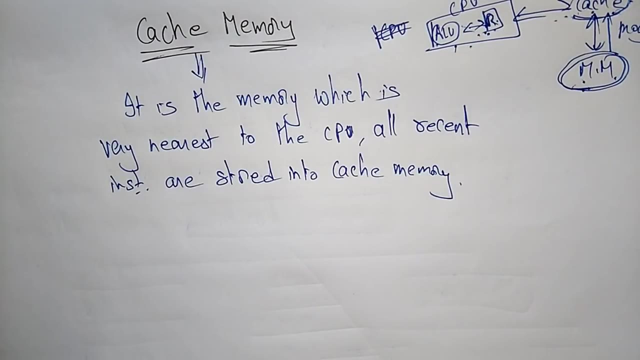 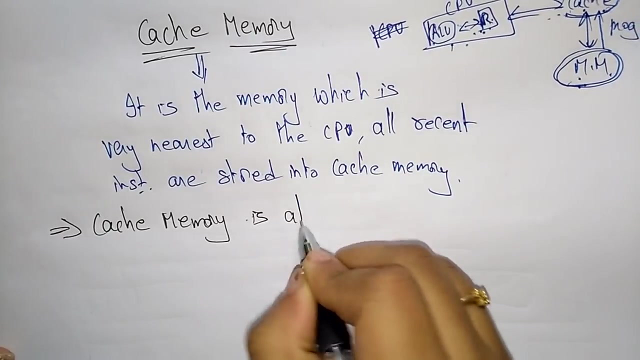 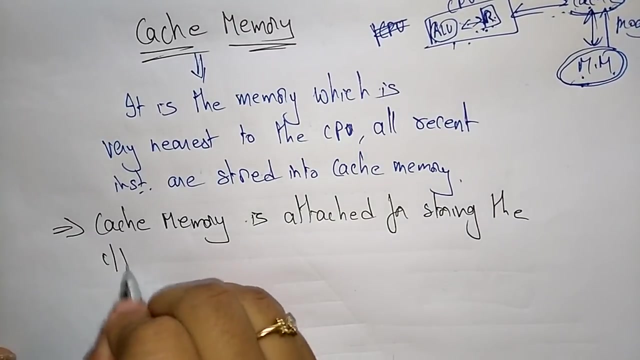 Instructions will be taken from main memory and stored it in the cache. So one by one the cache will send that information to the registers and from registers the ALU will take that instructions and performs the operation. So this is the cache memory. A cache memory is attached for storing. A cache memory is attached for storing the inputs which is given by the user. 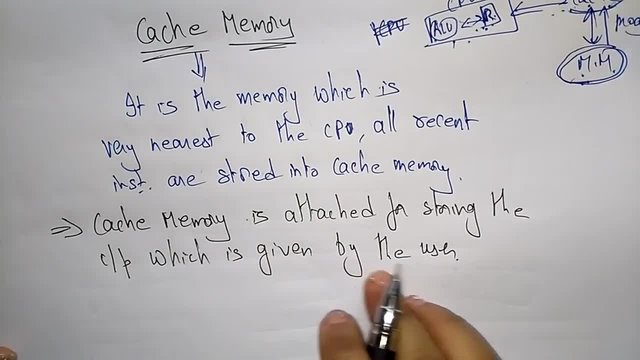 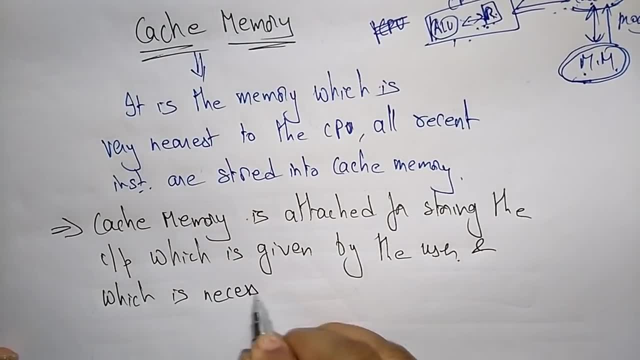 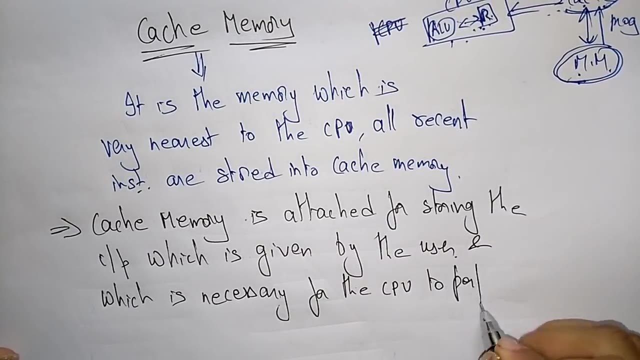 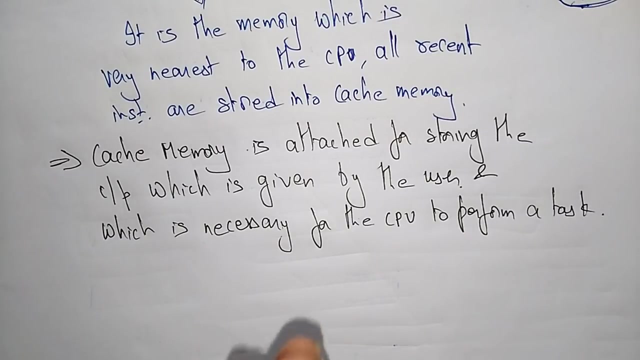 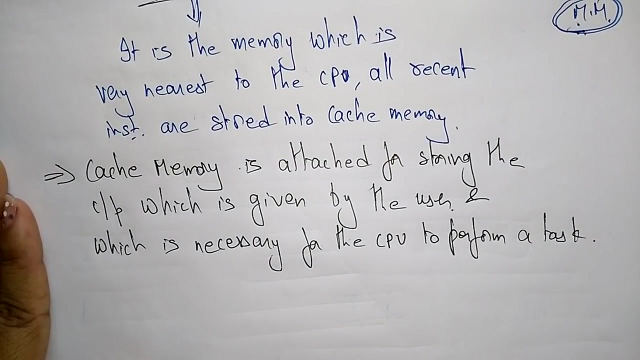 So the cache memory is attached for storing the inputs which is given by the user And which is necessary for the CPU to perform a task. So that is the operation that can perform by the cache memory. So cache memory lies in between the processor and the main memory, So it has less access time than memory and it is faster than main memory. 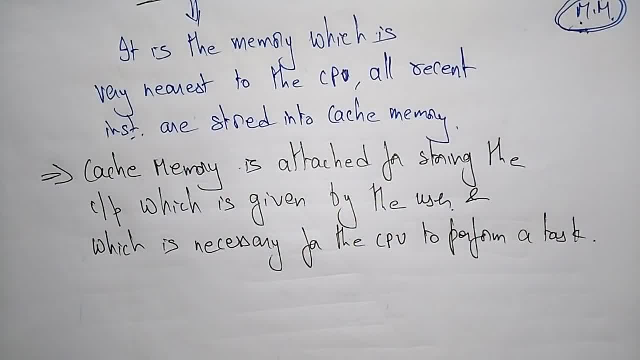 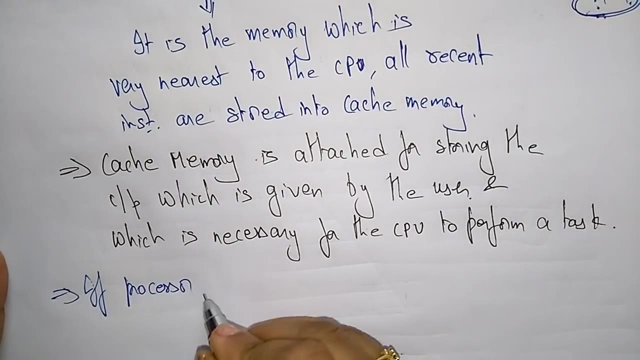 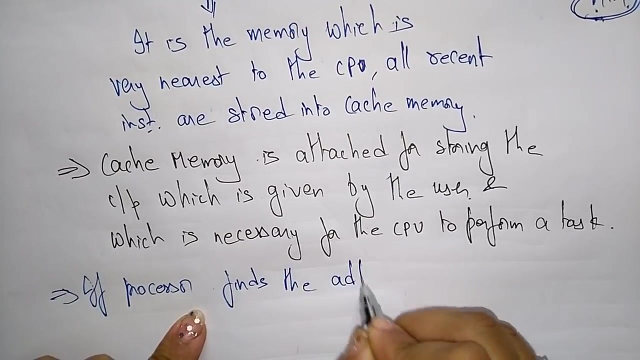 So the cache memory implements the cache logic and also if processor finds the address code or data is not available, Suppose let me write that. Suppose if processor wants to get some data from the cache, If processor finds the address code, It finds some address code. data is not available. 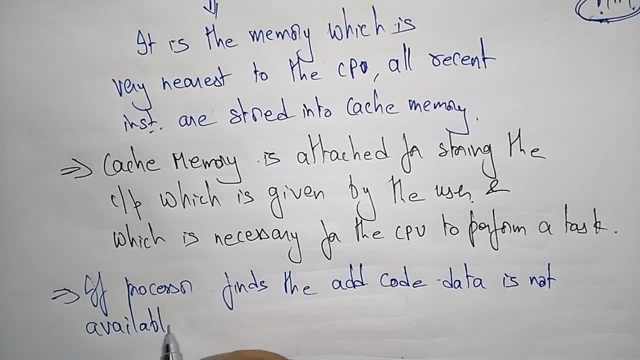 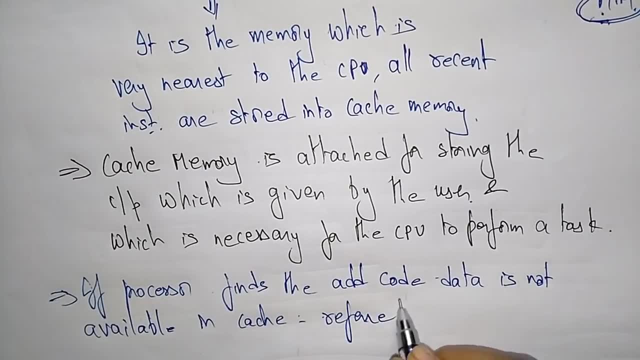 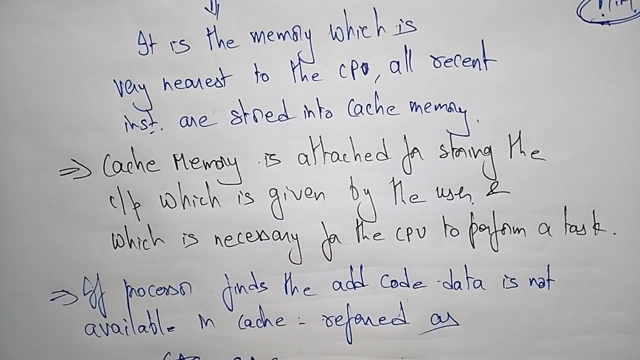 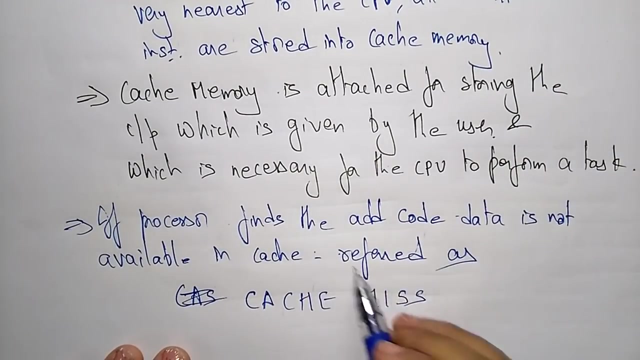 In cache. Suppose, whatever the data that the processor want, That data is not available in cache memory, Then it referred as cache miss. Sorry, C-A-C-H-E- Cache miss. Ok, So whenever the processor finds some address, code data So that data is not available in the cache. 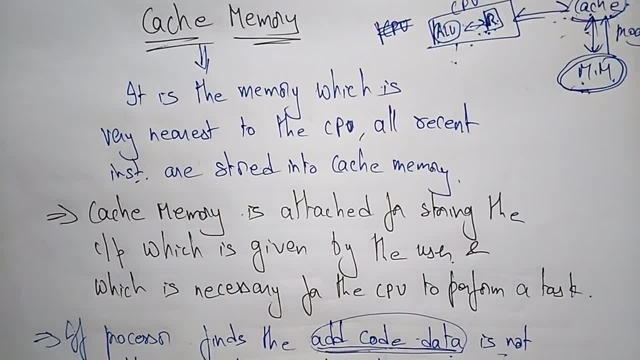 Ok, So whenever the processor finds some address, code data, So that data is not available in the cache. If the processor wants to execute some operation but that is not present in the cache, So then you call it as a cache miss, Cache miss. 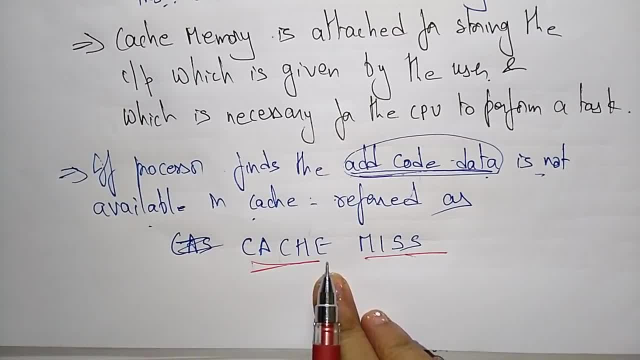 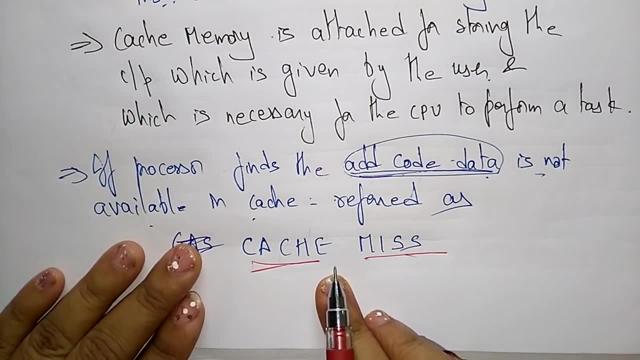 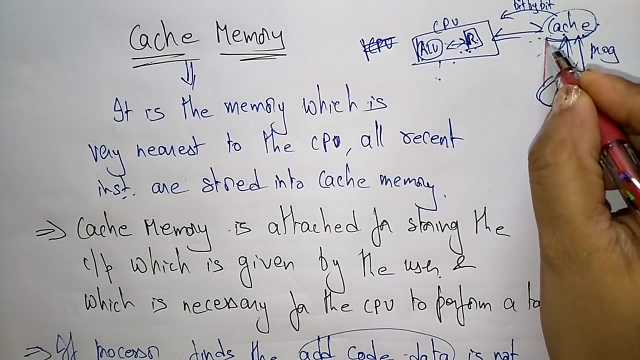 So if the desired memory block is, Then what it does, Then what the processor will do. if the data is not present in the cache, Then the desired memory block, whatever the processor want, that block is copied from main memory, Copied from main memory into cache. 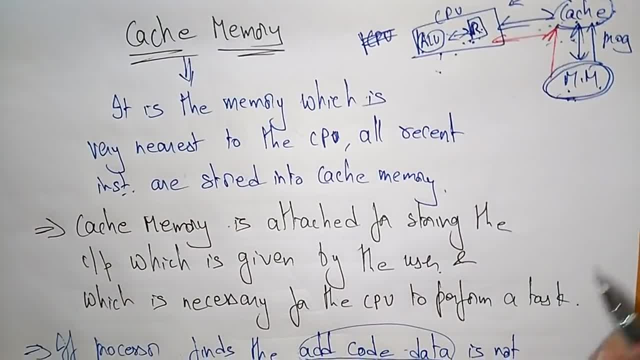 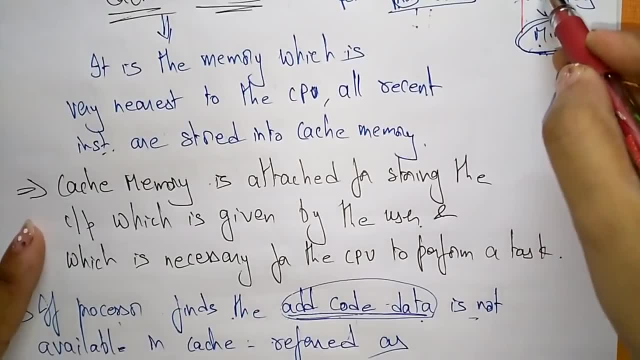 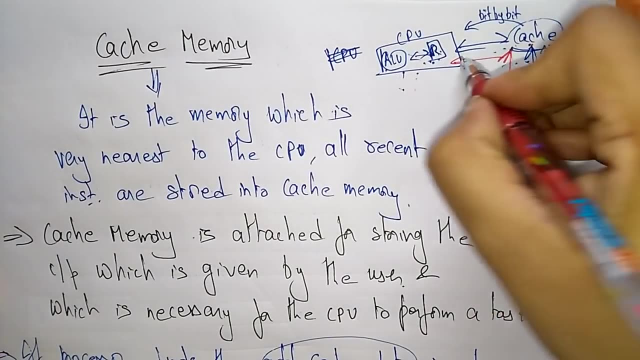 Using the cache control and sent to the CPU. Ok, So if the processor find something, if the processor want some data, if that is not present in the cache It referred to as a cache miss, Whenever the cache miss is occurred, The processor, the desired memory block, is copied from main memory, from main memory to cache, from cache to CPU. 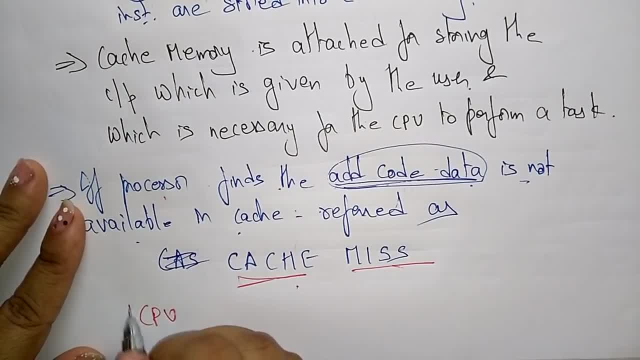 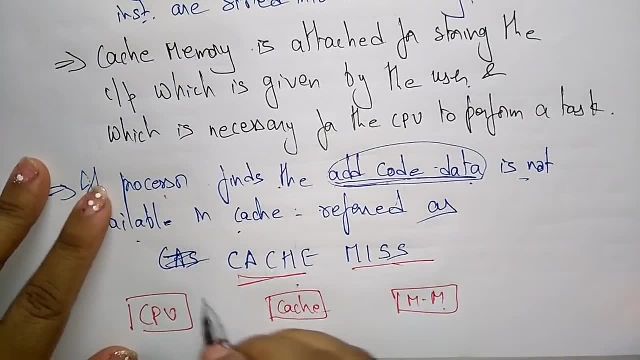 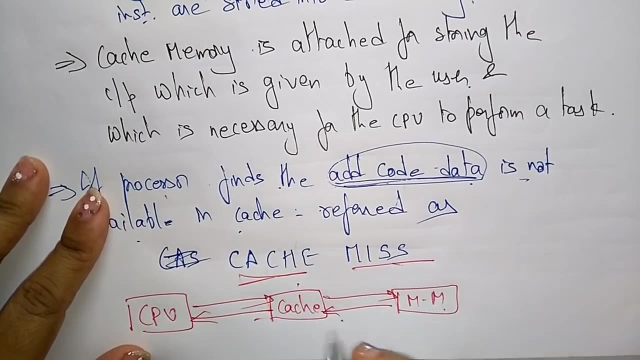 Ok, So this is how the data will be transferred: CPU Cache, Main memory: Ok, So The data transfer will be taken from cache to CPU And from main memory to cache. So this is how the operations are, I mean the data is transferring. 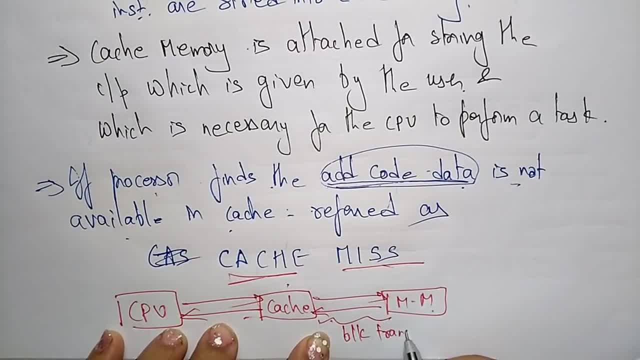 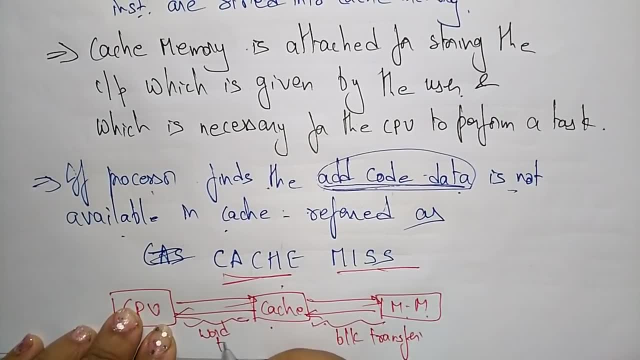 So here you call it as a block transfer. So block will be transferred at a time From main memory to cache, From cache to CPU. only word will be transferred, Word transfer. So here the transfer of bits will be word transfer. Where 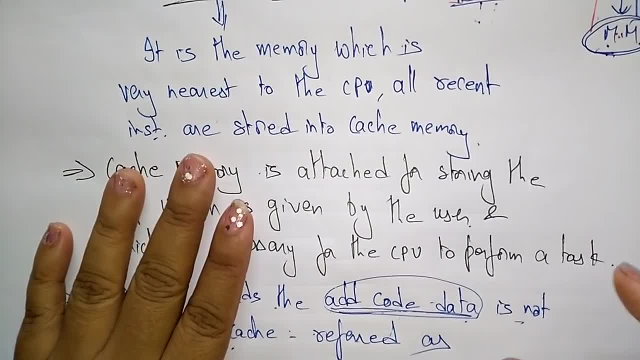 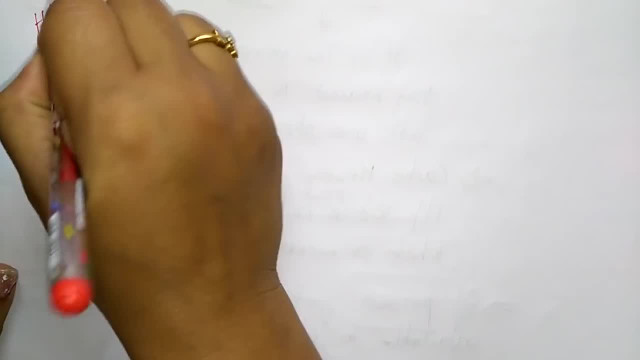 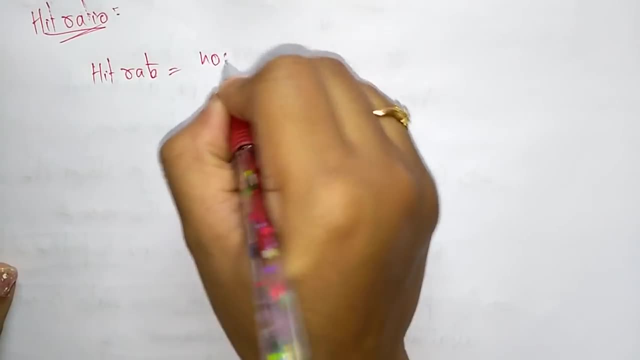 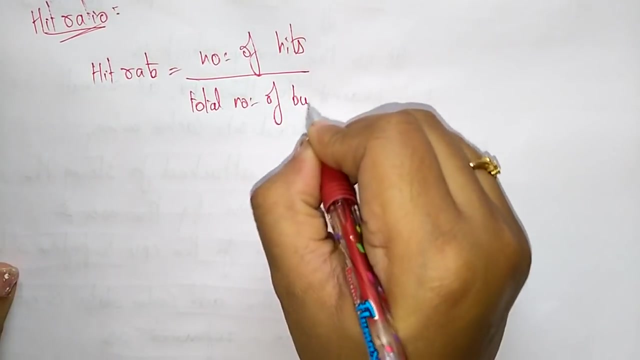 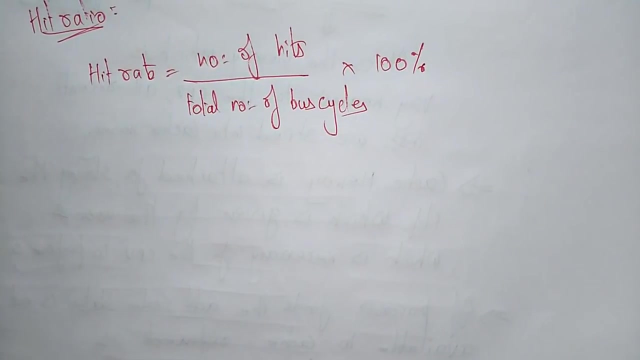 here will be the block transfer. So this is about the cache memory. So let me explain the formula for the hit ratio. hit ratio of the cache. So here the hit rate is equal to number of hits by total number of bus cycles into 100 percent. So this is a formula to calculate the hit rate. 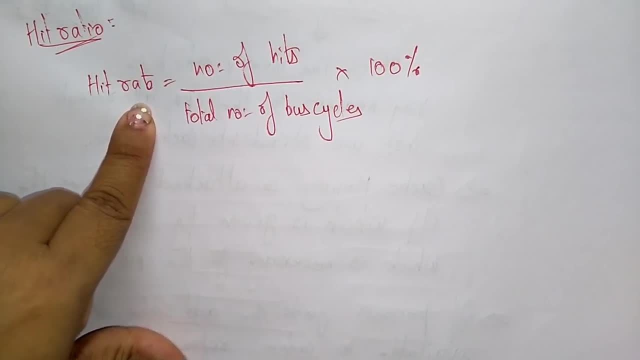 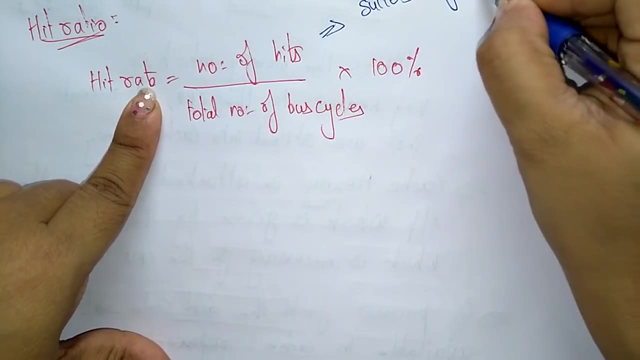 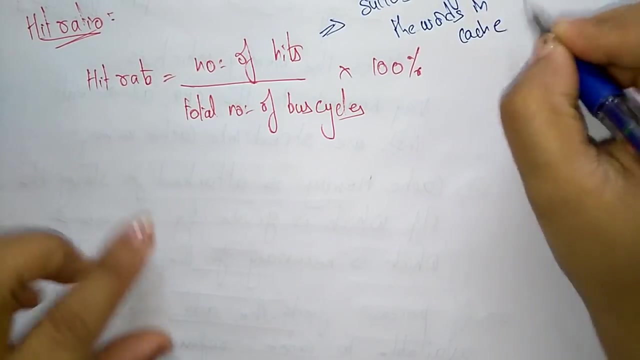 So what is this hit rate? Actually, this hit rate is used to calculate the number of hits. number of hits- nothing but success in finding the word, the words in cache. So number of hits is 100 percent. So this is the formula to calculate the hit rate. So